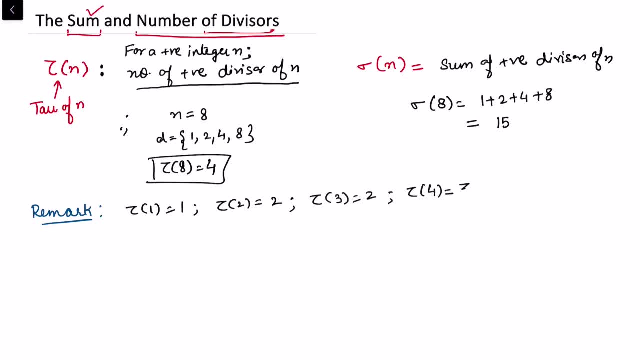 divisors of 3. Tau 4, there are 3 divisors of 4.. 1,, 2 and 4. Tau 5,: 5 is a prime, There are only 2 divisors and tau 6.. So for 6, we have 4 divisors: 1,, 2,, 3 and 6 itself, and the same list. 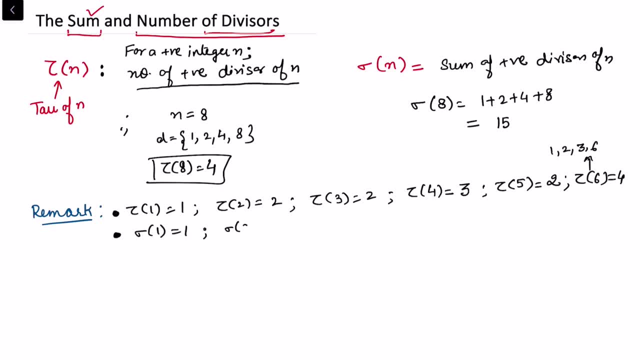 we can write down for the sigma also: Sigma 1 is 1.. Sigma 2, this is 3,. sum of the divisor Sigma 3, this value is again 4.. Sigma 4, this is 7.. Sigma 5, this is 6 and sigma 6 is 12.. Now, from the 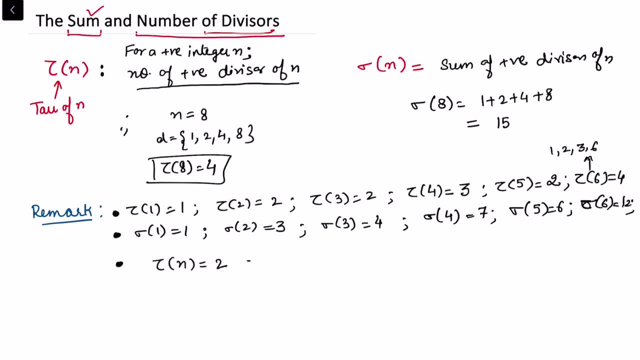 above example, it is very clear that tau n is always 2. if n is prime, We can see, because n is a prime and prime has only 2 divisor, 1 and n. So tau n is always 2 and same way sigma n. 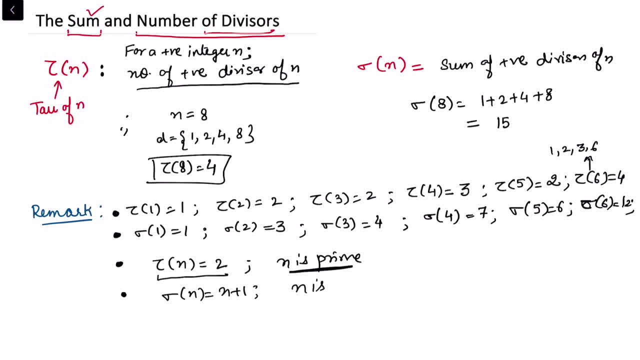 this would be always n plus 1. if n is prime, because the prime itself will come and then there will be one more number, which is 1, will always divide every prime. So this number is always n plus 1. and if we consider a representation of a function where summation f of d d divides n, 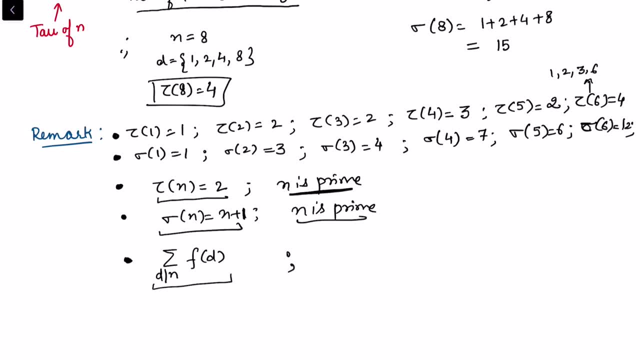 So this, in this representation we can always say: if I want to now write sigma n, sigma n is just the count of divisor, So I want to count divisor over n, So each time there exists a one added. So this is the expression in this form and similarly sigma n. Now I want to sum the 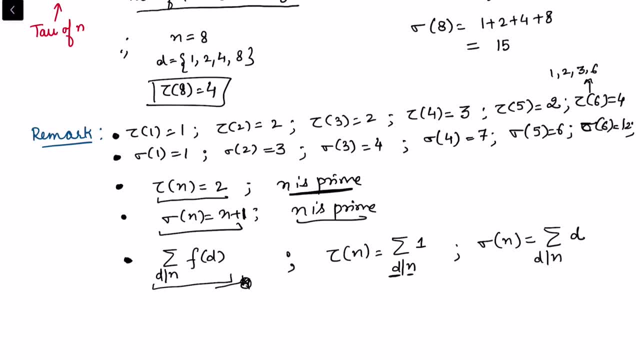 divisor, So summation over d. d divides n. So these two expressions are written in the arithmetic function form and again will be used again and again in the other properties of the sigma and tau n function. We can see the example of this above case. Let's take say, for example: 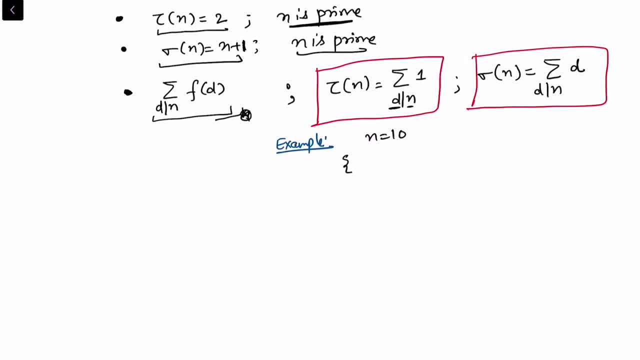 we want to consider, n is equal to 10.. In this case there are divisors for 10,, 1,, 2,, 5 and 10, and in this case, suppose I want to write tau n. This means d divides n. Now there are: 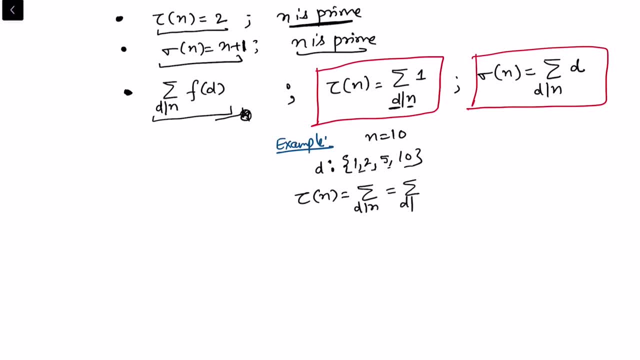 four divisors. So this means it is running over summation. d divides 10 and then 1.. So sum over all divisor. when d is 1, it will take one value. When d is 2,, it will again take one value. When d. 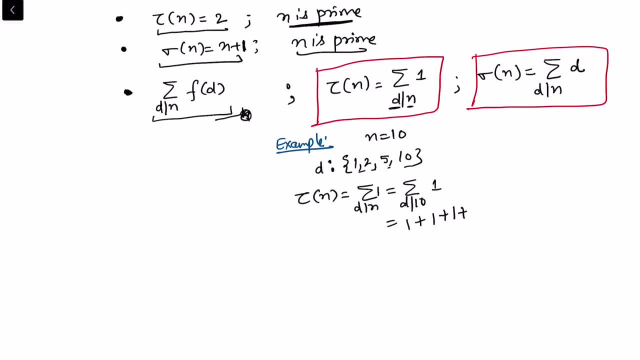 is 5,, this will again take one value, and when d is 10,, this will again take one value. So that tau n is 4, and similarly for sigma n. Now, if I want to count sigma 10,. this is summation. 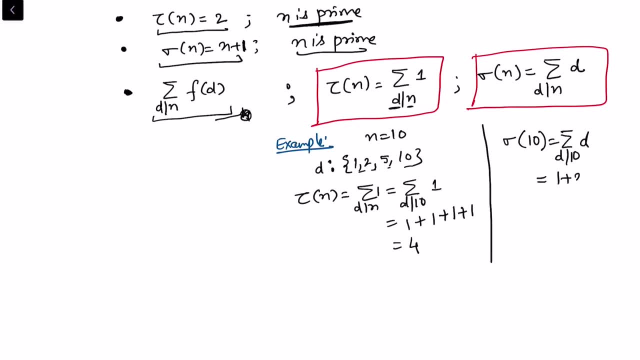 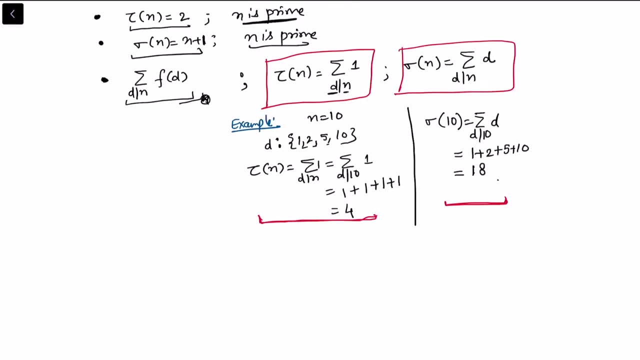 d divides 10 d and similarly, when I run now summation over the divisor, this will give me this quantity and in this case this will give me 18.. Now for smaller value. it is easy to write down this divisor set, Say, for example: now I consider a larger number, Let's take here a larger 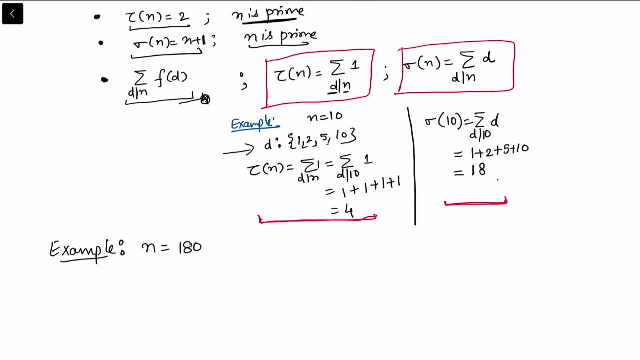 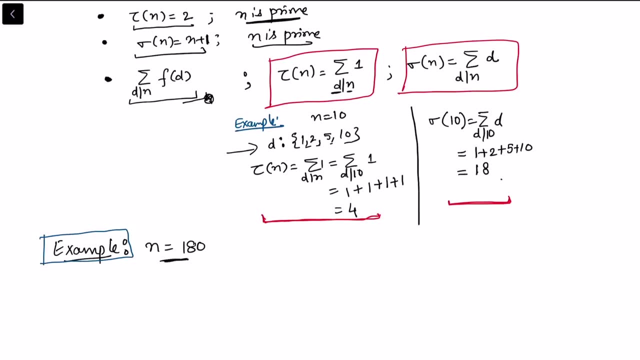 number, as n is equal to 180.. Now I want to list down all the positive divisors of 180, and so I want to compute what is tau n. So now, if I look at the number, n is equal to 180,. 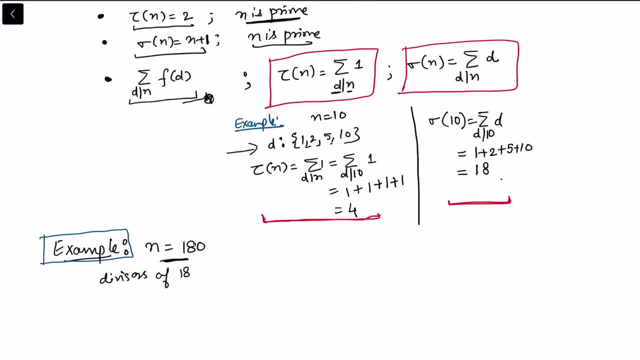 divisors of 180 are. we can list out this one: 1,, 2,, 3,, 4,, 5,, 6,, 9 and so on. There are many divisors, So it is difficult to write all this list. So what we are searching is: is there a? 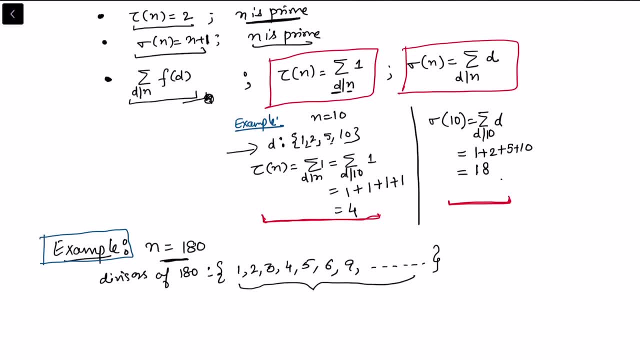 way to find the divisors and then, once we know the divisor, we can then sum the divisor to find what is sigma of 180, and earlier we were talking about count on divisor. That means we need to know what is the formula for count on divisor. So we need to know what is the formula for. 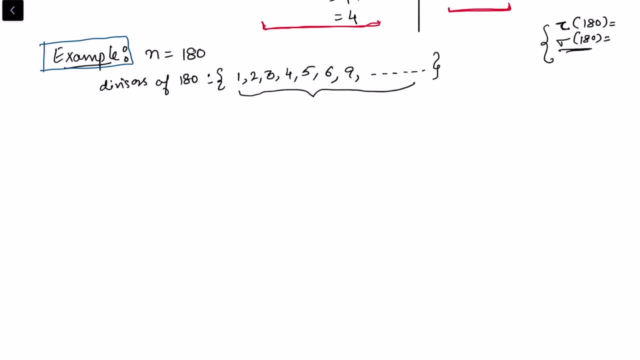 this way. So to know the formula of tau and sigma for the general value of n, let me to write n as the prime factorization, So in this case n is 180.. Let's write down this into the prime factorization: 2 square, 3 square into 5, and from there I want to know what is the divisor of n. 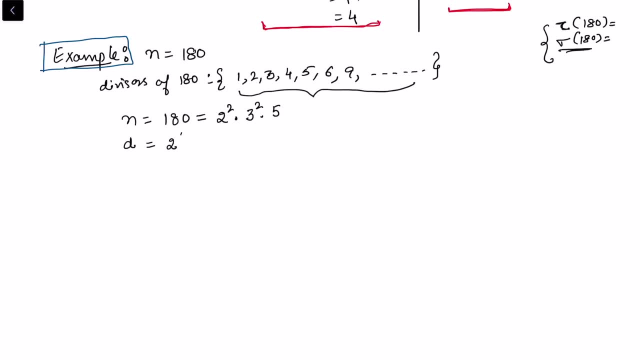 So divisor also take the same prime factorization. This means 2 to the power a1,, 3 to the power a2 into 5 to the power a3, where there is a restriction on these. a i's So 0, a1 lies. 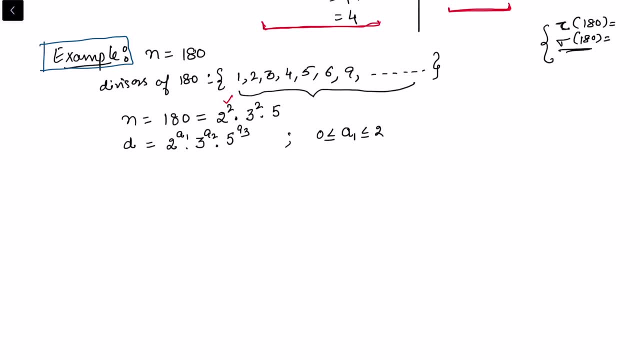 0 and 2 because of this power here, because 2 can come maximum with the power 2 in the main integer, and similarly a2, which is the power of the second prime in the divisor. a2 can go maximum again till 2 because of this 2, and a3, which is the power of 5, here that has a 1 power in the main integer. 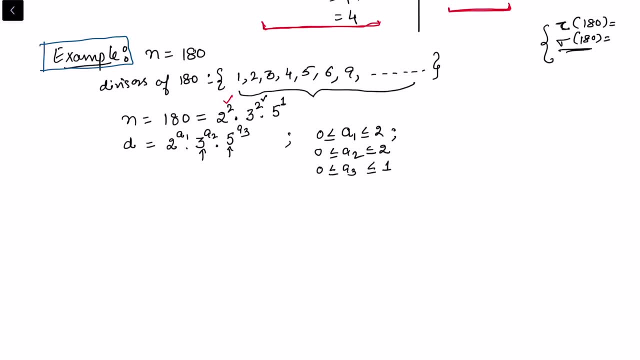 So 0 less than, a3 less than or equal to 1.. Now, taking different choices of this d, we will get the divisor. So, for example, I will take a1, a2, a3 as all 0. So let's keep this as 2 to the power 0, 3 to the power 0 and 5 to the power 0.. 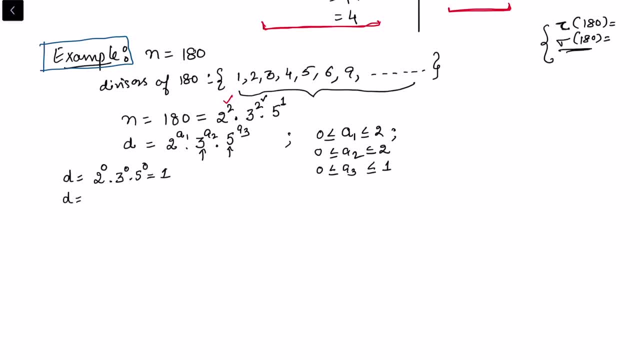 This is 1, because anything raised to power 0 is 1.. If I now take any other choice, suppose 2 raised to power 1 I take, and then I take all other combination of 3 raised to power 0 and 5 raised. 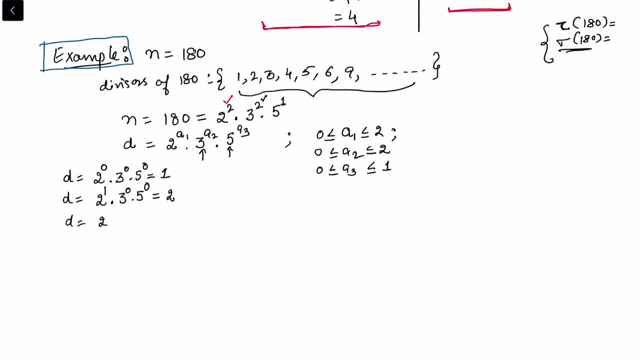 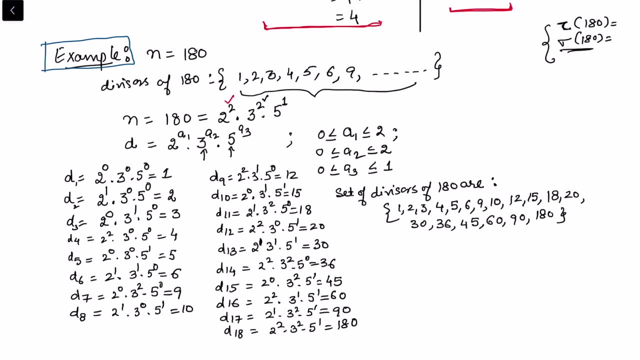 to power 0. This will give me 2.. If I now vary my combination- 2 to the power 0, I will take 3 to the power 1 and 5 raised to power 0. This will give me 3 and so on. So we get: there are 18 such divisors. 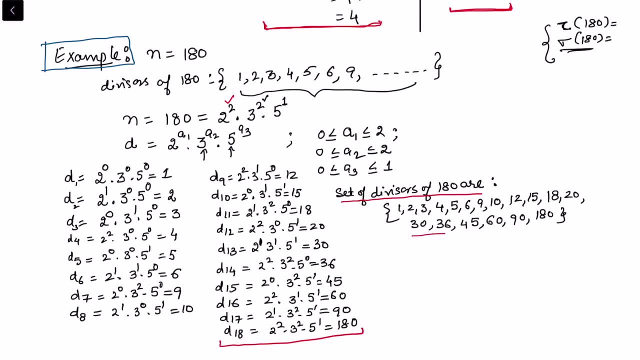 And here we have written now the set of divisor of 180 are this: So by taking the same prime factorization in the divisor and running over the choices of a, we can get all possible divisor. So this implies tau of 180. simply by looking at the count of all these possible divisor, 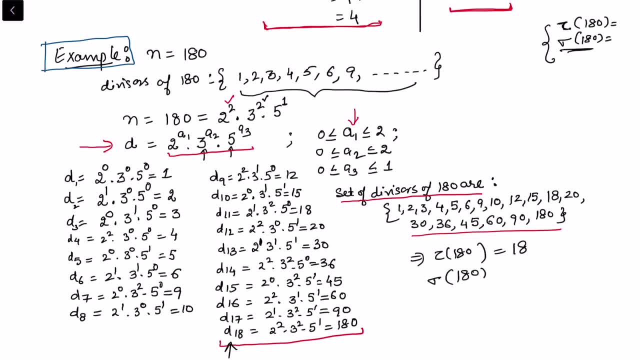 this is 80.. And from here we can see sigma of 180.. Now some these divisor that I have got in this particular set will give me sigma of 180. But again, summation is difficult. count was little easy to find it from here by taking the different. 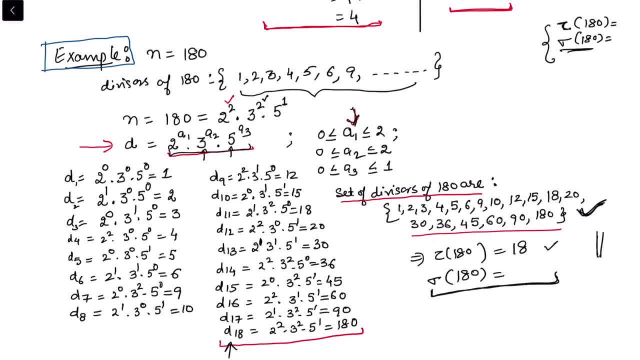 combination. So now we will be doing a theorem that allow us to know what is a formula for tau 180 and formula for sigma 180 in general, based on the prime factorization that appear in the integer n. So the first thing that we prove now is that whenever n has a prime factorization of 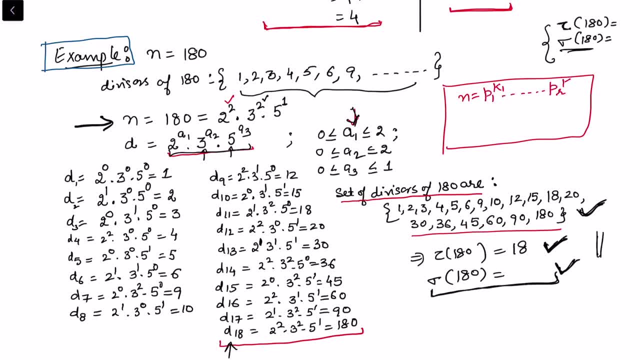 the form p1 to the power k1, pr to the power kr, then we say: if d is a divisor of n, then d must also take the same form, p1 to the power a1, up till pr to the power ar, Where each of this ai lies between 0 to ki. So this is the fact that I have used. I have used. 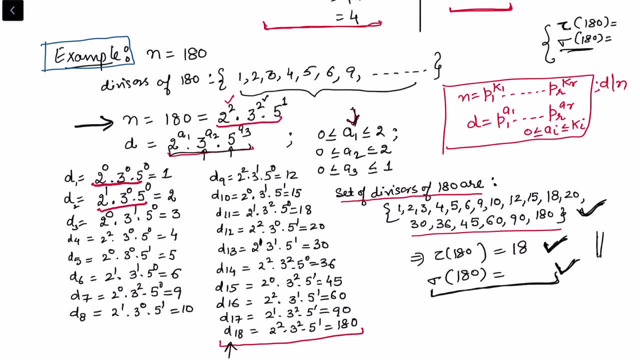 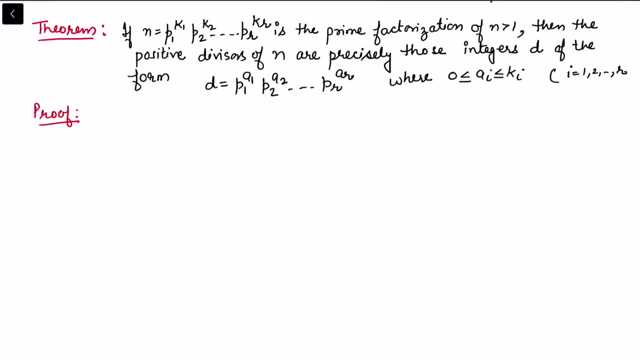 the same prime factorization that appeared in the integer, And here I have varied the power of ai's maximum till the ki that appear in the integer n. So let's first prove this result and then we will proceed for the formulas of sigma and tau n. In this result we want to prove 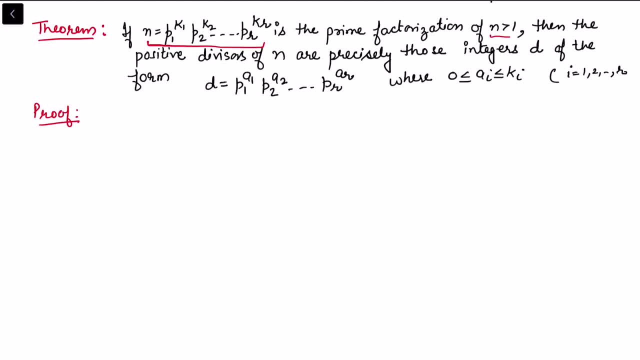 if n takes this prime factorization and n is strictly greater than 1, then what are the divisors of n? d will also take the similar form and here, if the power ai is, will always be less than or equal to ki And of course the least value of ai can. 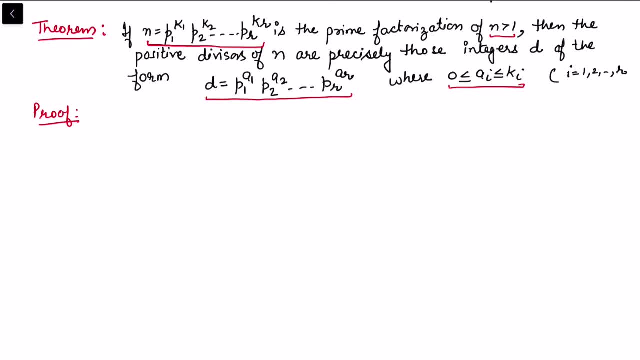 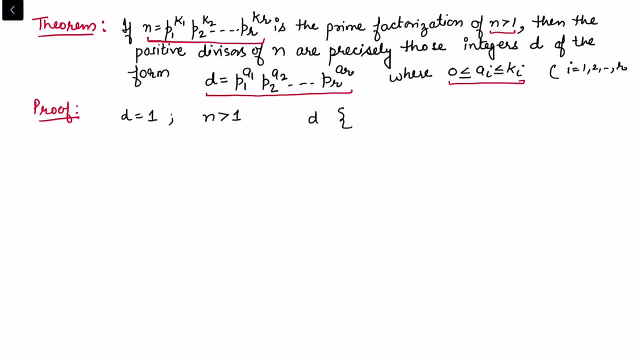 be 0. Now let us prove this case. So suppose that divider did is equal to 1, we know that n is greater than 1.. So n have a list of divisor, and divisor can be 1 and itself, And 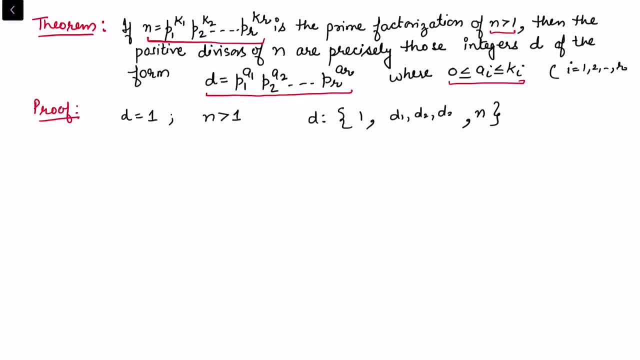 then there are some proper divisors. okay: d1, d2, d3.. So these are proper divisors. So let us take when d is equal to one, so d2 get equal to one, So the rest of las divisors can be equals to two and N can be equal to n. So 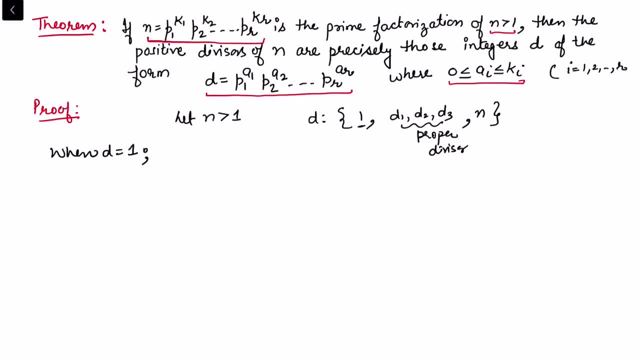 let us break this down from here. so d1 get equal to 1 in sum, when d is equal to 1, so when d is equal to 1, this is only possible when a1, a2, all powers, this is equal to 0 and in this case, left condition hold true, because we are claiming that ai can. 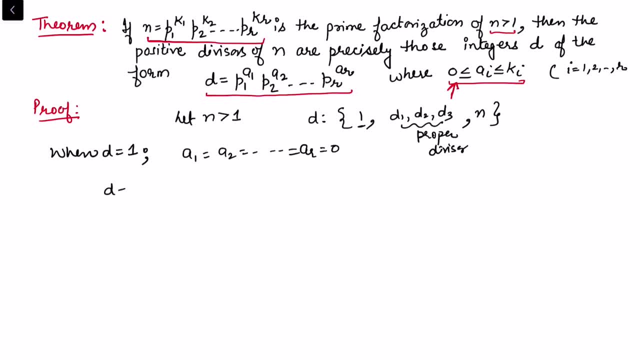 take the least value as 0. take the other case, when d is equal to n. so in this case, take a1 equal to k1, take a2 equal to k2, and so on. ar equal to kr. so in this case, as the power ai, take the. 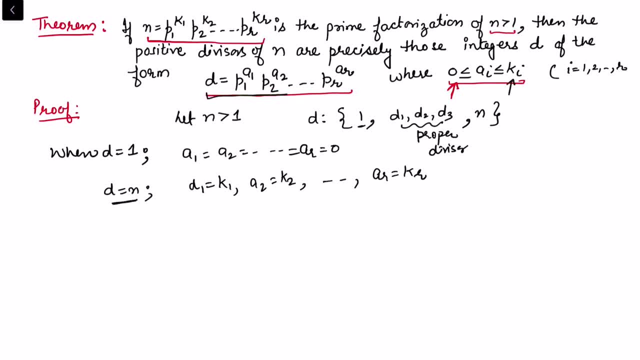 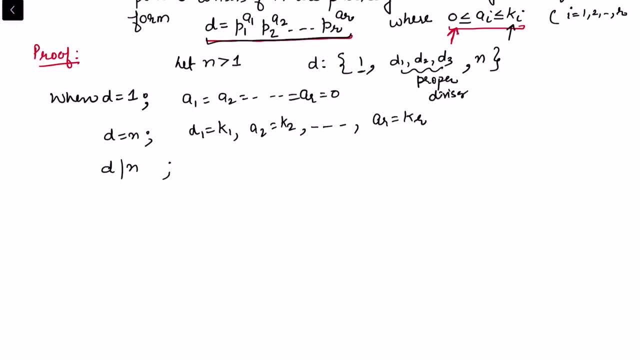 maximum power, d automatically become n, so that the prime factorization of d and n- they are exactly same, which is the case. and consider the case when d is strictly dividing n or it is a, d is a proper divisor of n. in this case i can write n as d into d dash and both of these quantity, d1, is also greater. 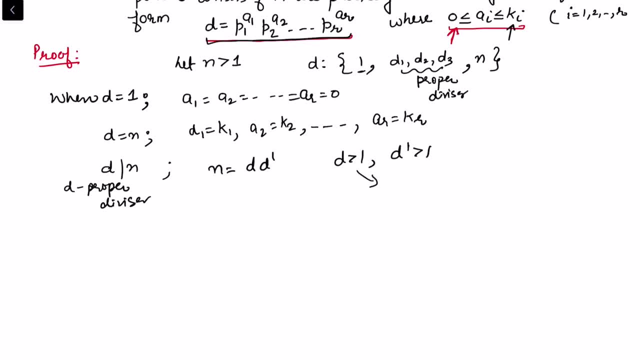 than 1 and d dash is also greater than 1. let us write: d also has a prime factorization, because whenever a number is greater than 1, we can have by fundamental theorem of arithmetic that every number can have a prime factorization of n and d dash is also greater than 1. so in this case, 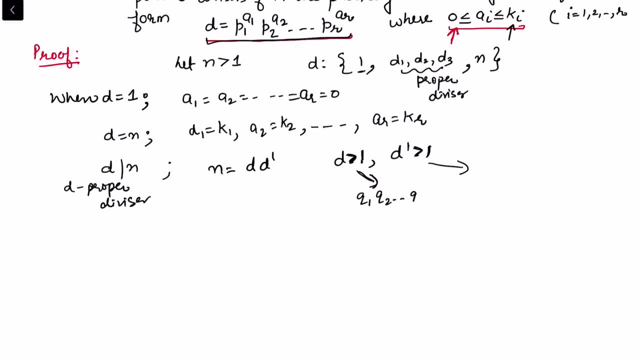 we can have a prime factorization. so let us write q1, q2 up till qs. and for this also i am going to now write a prime factorization: t1, t2, not necessarily distinct. say, for example, i have consider n as 24 and i can write this as 2 into 12. now 2 has a prime factorization. that is 2 only. 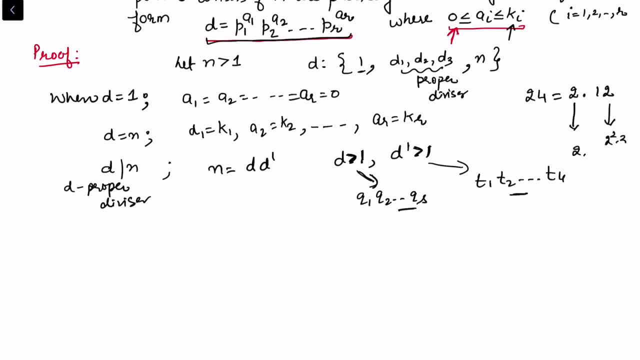 but 12 can have a prime factorization that is 2 square into 3. so this number 2 is repeating in the 2. so here i can write this as d and this is d dash. so there are some primes which are repeating on this expression. we have taken n as the prime factorization, which is p1, k1, up till, so on pr kr. 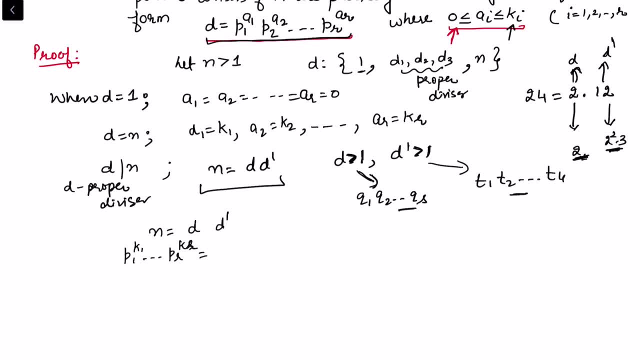 and we are writing this as d into d dash. so this means d is q1 up till qs and d dash is t1, t2 up till tu. now in these prime factorizations some of the prime factor may repeat. so collecting the equal primes, collecting the repeating primes on the right hand side, repeating primes on right. 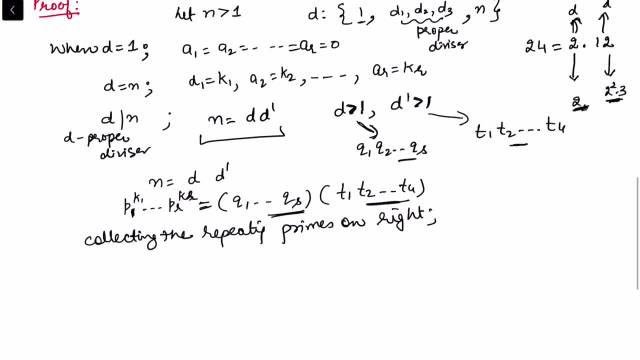 hand side, and on the left hand side, and on the right hand side, and on the left hand side and on the right hand side expression. what we get is that d can be written as definitely in the form of p1, because on the left hand side we only have the base prime as p1 to pr. so obviously, 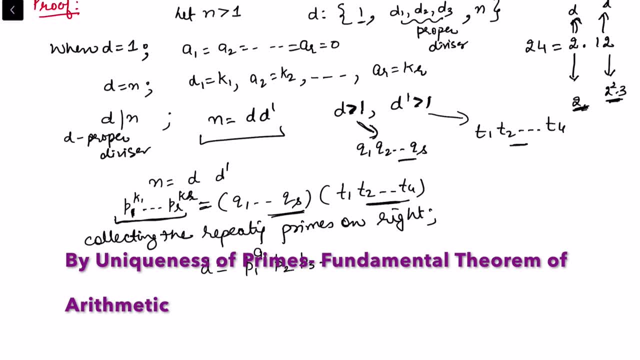 d will also have p1, p2, p3 up till pr, if there is any other prime, and then this is equal to the multiplication of the right hand side. that is not going to possible. so we have a1, a2 up till a3, up till ar, and of course these ai may be greater than or equal to 0, but the maximum value is of course 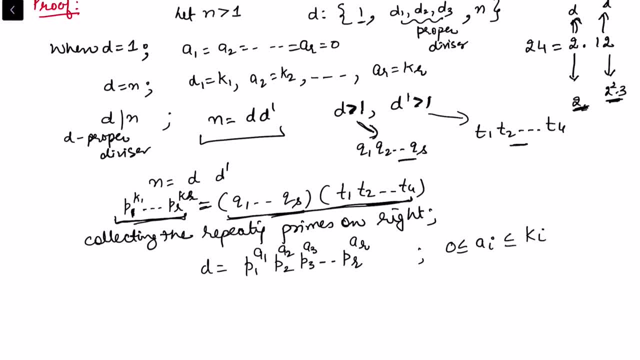 up till ki, and conversely, we can also write that every member of d, when it's selected into this form, p1, p2, a2 up till, so all pr? ar. i can write down n as p1, a1 up till pr? ar and then remaining quantities are: 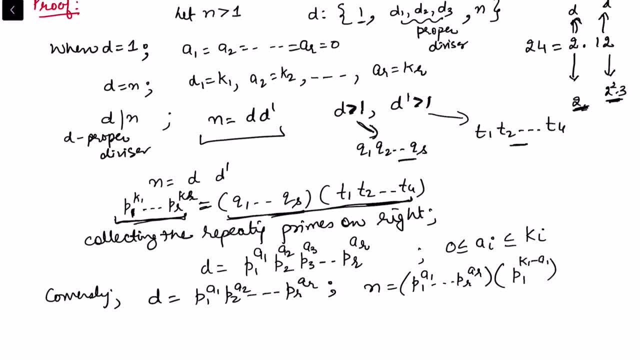 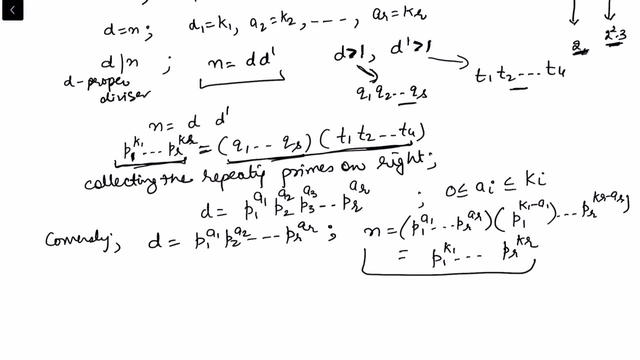 subtracted from here, p1 minus this and so on, pr kr minus ar, so that the total product will become back to k1, and that is the prime factorization that we have taken it for n. so that ensures that whenever there is a d which is acting as a divisor of n, so this divisor will also take the same prime. 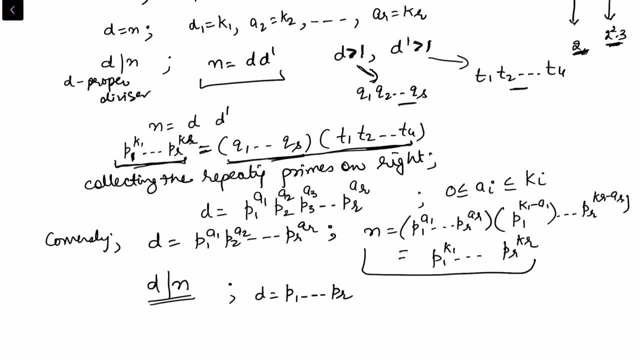 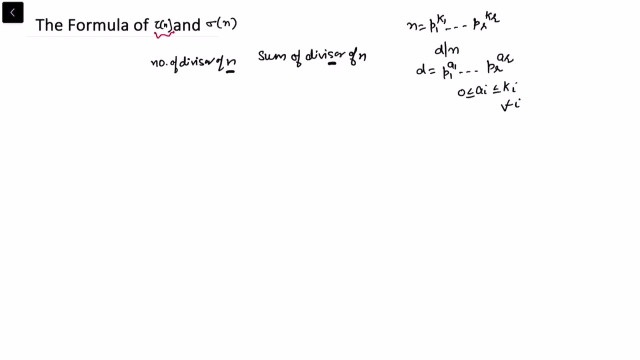 factorization, which is appearing in the n. but the possibility for these power is that they can be 0 or they can be less than or equal to ki, but they will not exceed the powers that is appearing in main integer n and hence that result. Finally, we find the formula for tau n and sigma n. this is number of divisors of n and sum of divisors. 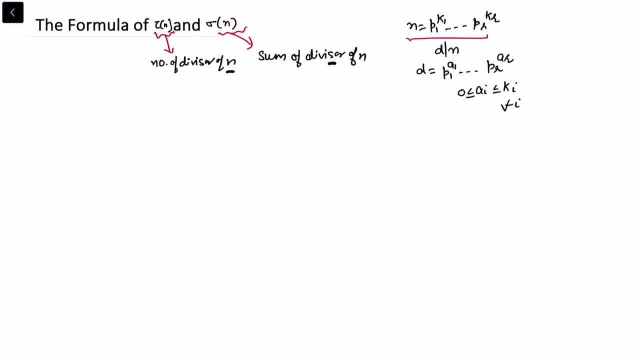 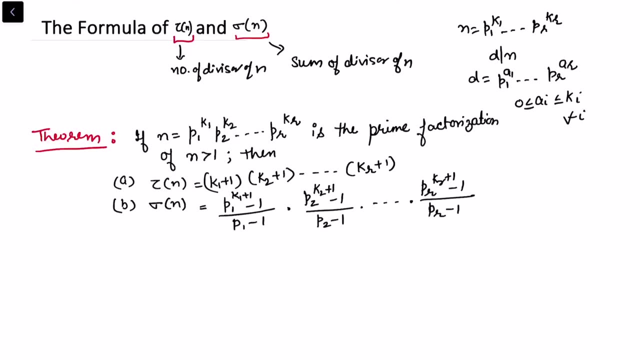 of n. and we know, whenever we have n as this prime factorization and there's a d dividing n, then d also takes prime factorizations. so the theorem state of n is in the prime factorization p1 to the power k1, up till pr to the power kr. then tau n is given by this expression and sigma n is given by: 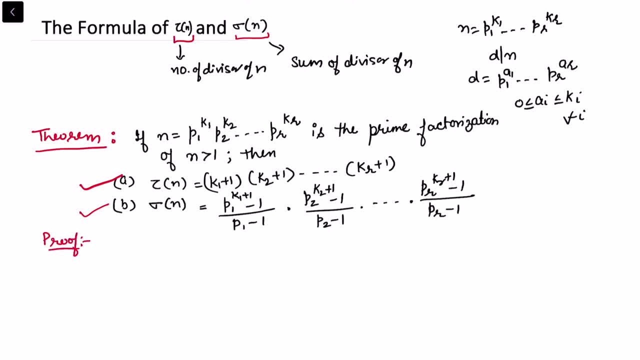 this expression. Now let's prove this result, and in the proof I'm just going to consider the prime factorization of n and its divisors. factorization of n and its divisor. so we have been already given that the prime factorization of n is this so obviously positive divisor d of n will take this form: p1 up till pr. and these ai's lie. 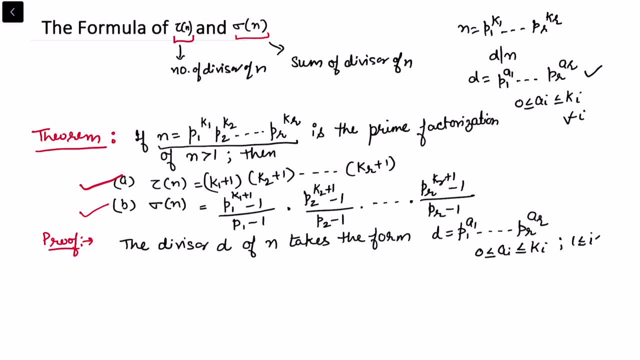 between less than or equal to ki and i, varying from 1 to r. as we have just discussed. we have proved this theorem in the last video. now we can see how many possible choices for a1 do we have, because we want to count how many divisor of d of n can take place. so that will be giving me the. 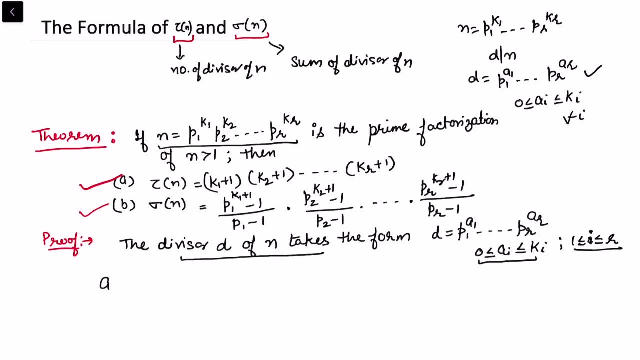 value for tau n a1 can take. this can take k1 plus 1 value because ai varies from 0 to ki, so from 0 to ki it has a1, takes k1 plus 1 value. so that means let's see here 0 less than or equal to a1. 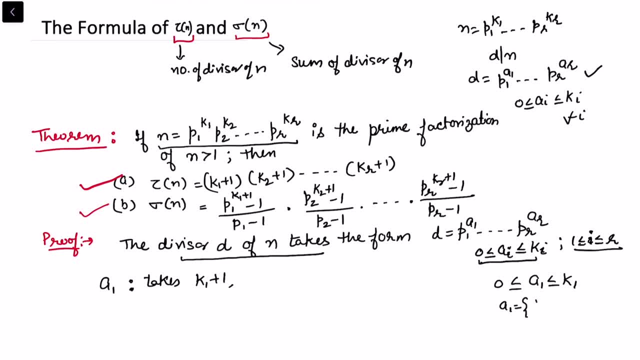 less than or equal to k1, so a1 can take the value. either a1 can be 0, or it can be 1, or it can be 2, up till it can be 1. how many numbers do we have the possibility for a k plus 1 number? 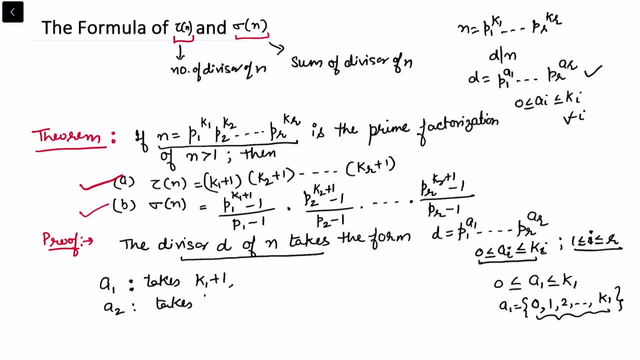 similarly, a2 can take k2 plus 1 and so on. ar can take the possible values as kr plus 1, and these are the possibility of the divisors, because in each divisor, d, we can have either the prime p1, or we may have p1 into p2, or we may have the other prime, factorization. so the total number of the 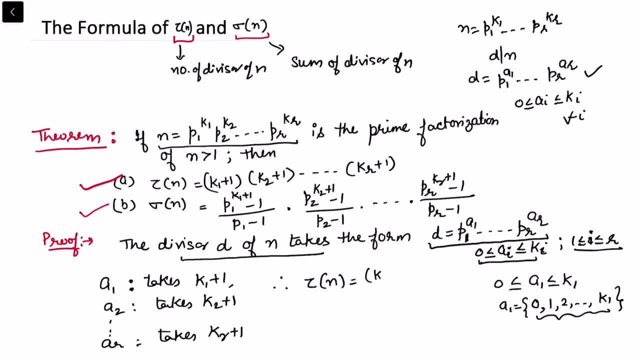 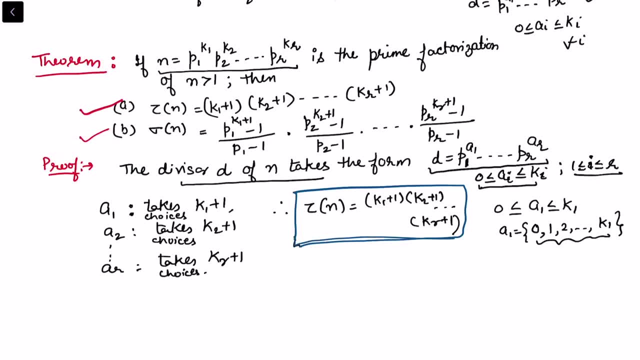 possibility for tau n. this is the k1 plus 1 into k2 plus 1, multiplied by kr plus 1. so this proves tau n case and hence i have proved now the first case. now, in this second case also, we will continue the same investigation as a1 takes. 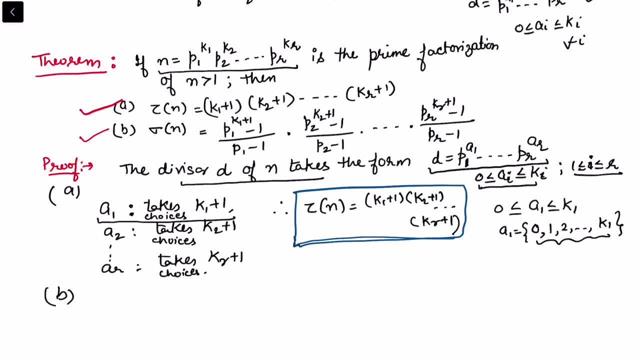 k1 plus 1 choices. so here i want to now sum the divisor, because in the sigma n the definition is the sum of the divisor. so for example, the first divisor whenever d divides n, the first possibility of the summation is when p1 to the power a1 will come. so 1 is a divisor and the sum of the divisor 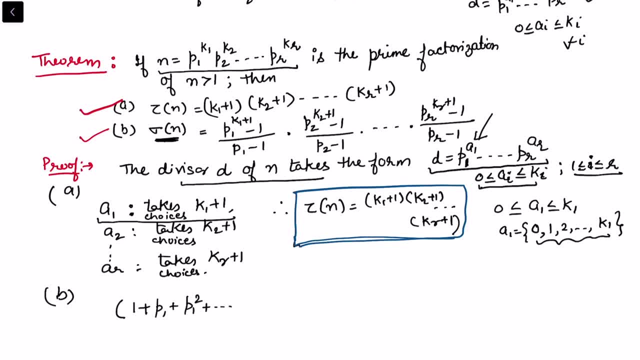 p1 is a divisor, p1 square is a divisor, and so on. the last term in the first divisor is p1 to the power a1. so we have summed all these divisor. it has this much possibility. and then we have the another possibility, p2, up till so on, p2, a2- this is the possibility for the second case- and so on. 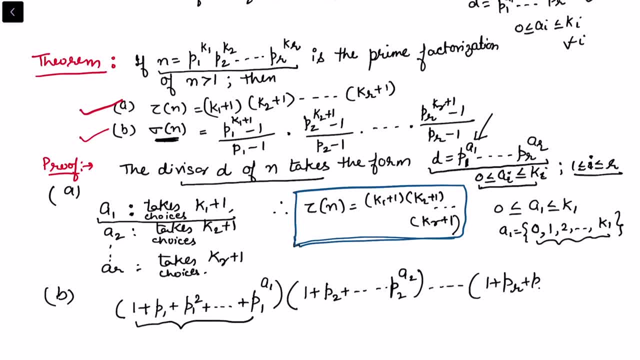 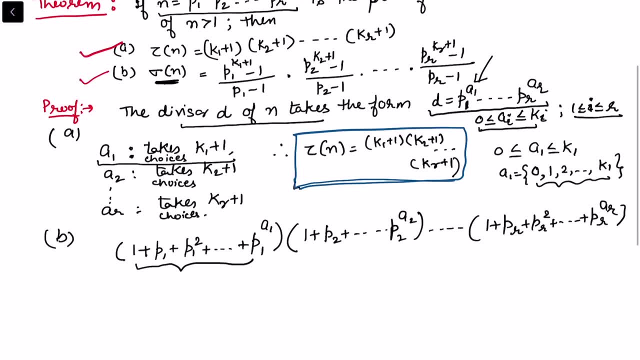 we are summing now. the last case: pr, pr square, and so on up till pr, to the power ar. now we know that this summation is a gp, and in this case we have the common ratio as 1, p1. here the common ratio is p2, here the common ratio is pr. these are finite gp, and so to write sigma n, i'm just using the gp. 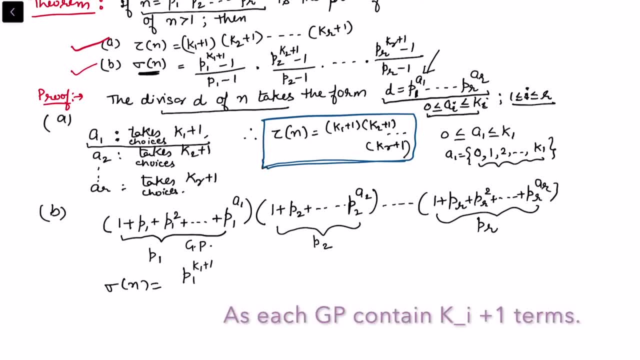 summation formula and this will become p1 to the power- k1 plus 1 minus 1, p1 minus 1, and we will be using this r minus 1 form because we know that the prime is strictly greater than 1. and similarly, for this expression i will use p2 to the power: k2 plus 1 minus 1 upon p2. 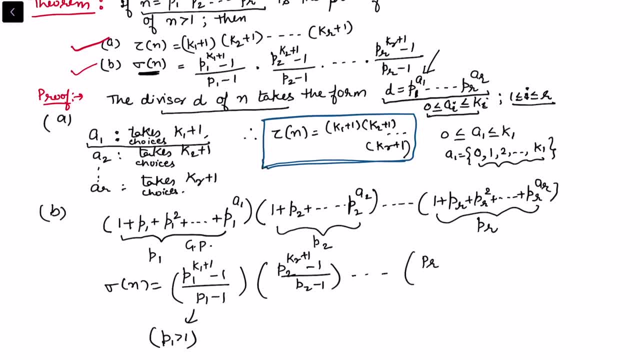 minus 1, and so on: pr to the power, kr plus 1 minus 1, pr minus 1, and hence the expression to also hold. so here, in the first case, it all depends upon the choices of the divisor, and we can look at from the individual choices, and here we can simply count that and in the next formula we can sum that. 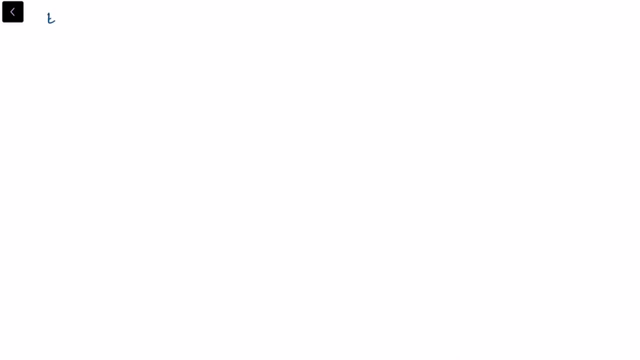 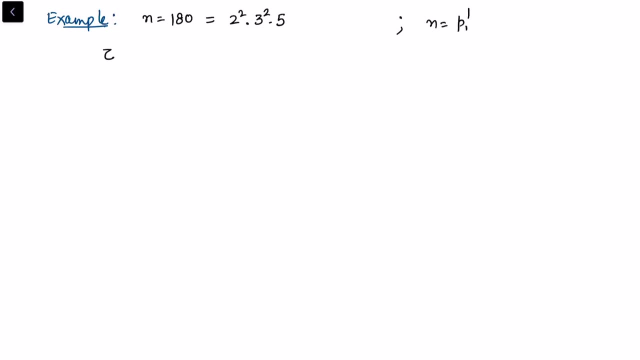 the formula say: if n has the prime factorization p1, k1 up till pr to the power kr, then tau n is the k1 plus 1. so whatever be the primes power k1, just add one more. we have just seen in the proof, and this is kr plus 1 and sigma n, this is p1 to the power, k1 plus 1 minus 1 upon p1 minus 1.